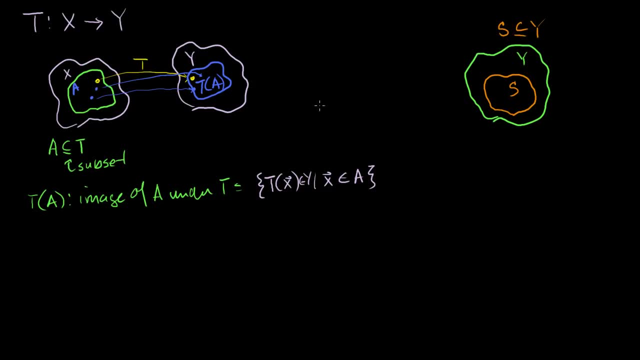 So s is a subset of our codomain y, And I'm curious about what subset of x maps into s. So I'm curious about this set, I'm curious about the set of all vectors that are members of my domain, such that their mapping or the 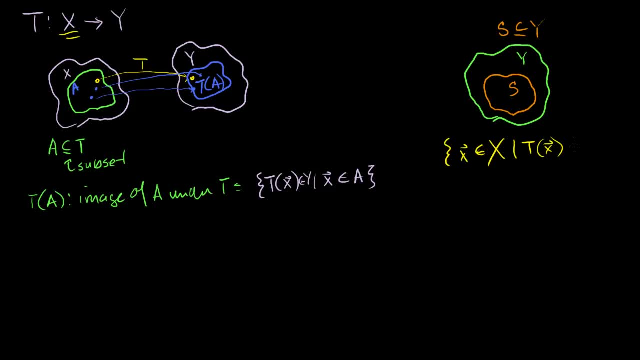 transformation of those vectors ends up in my subset of s. So what I'm saying is: look, if I take my domain, there must be some subset of vectors right here where, if I take any member of this set, it will map into these guys. 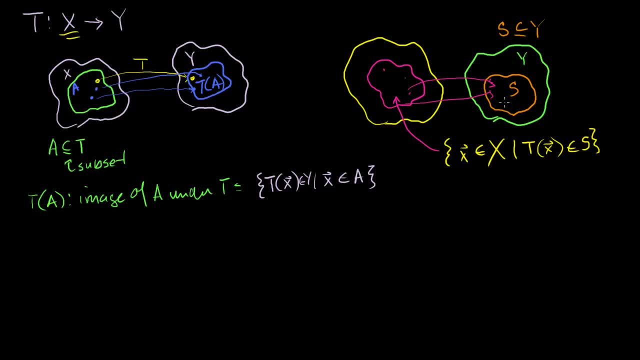 And that's what I'm defining right here. This is equal to that guy. So I'm literally saying OK, OK, What is? are all of the members of x? where those members of x all map into s? Now I want to make a very subtle nuance here, or point? 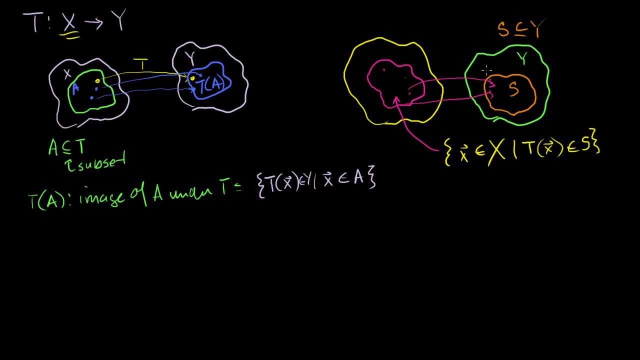 out something here. I'm not saying that every point in s necessarily gets mapped to. For example, maybe there's some element in s right there that no element in x ever gets mapped to from our transformation t. That's OK. All I'm saying is is that everything in this set maps to. 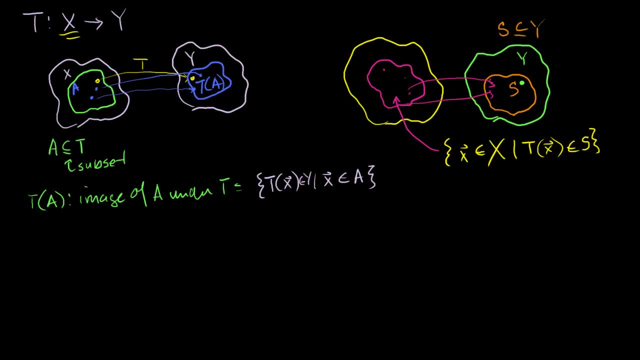 something, Something within s right here, And what we call this, we call this set right here. we call this: the notation is the inverse t of s, But this is equal to the preimage of s under t, So this is s. 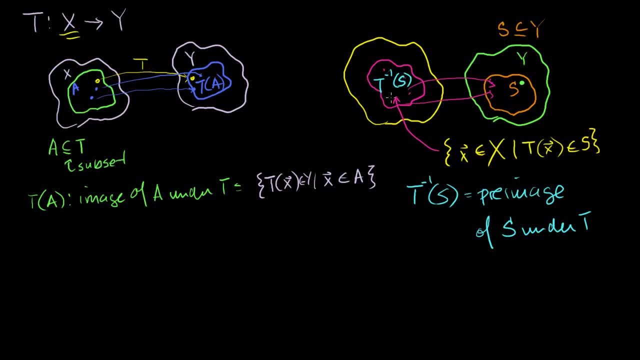 This is the preimage of s under t And that makes sense. The image: we go from a subset of our domain To a subset of our codomain. Preimage: we go from a subset of our codomain And we say what subset of our domain maps into that subset. 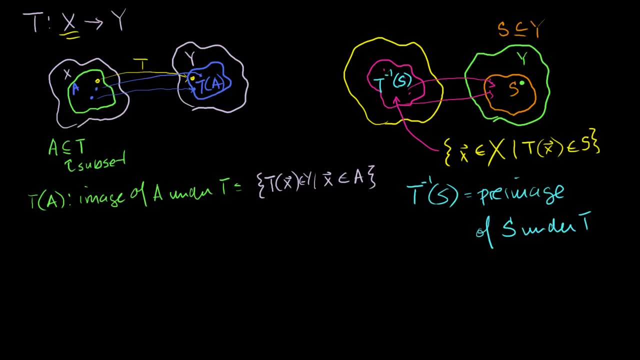 of our codomain. Now let me ask you an interesting question, and this is kind of for bonus points: What is the image of our preimage under s? So what is the image of our preimage under s? So if we take this guy, the pre, this is essentially